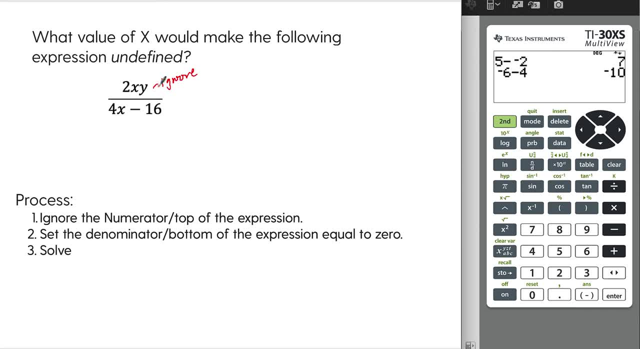 ignore this part. It doesn't matter what it is, how gnarly it is or how simple it looks, Just ignore it. Then this whole thing here: this 4x minus 16, you can set that equal to zero and then solve for it. You can do plus 16 on both sides. 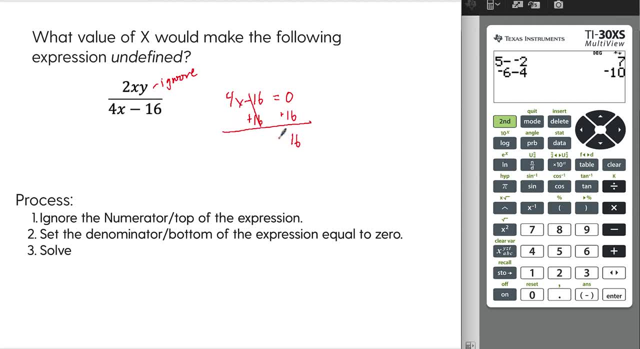 Okay, these are going to cancel out. You'll end up with 16 equals 4x, And then you divide by 4 to isolate x And you're going to see that x equals 4.. So, in other words, when you get 4 times 4,. 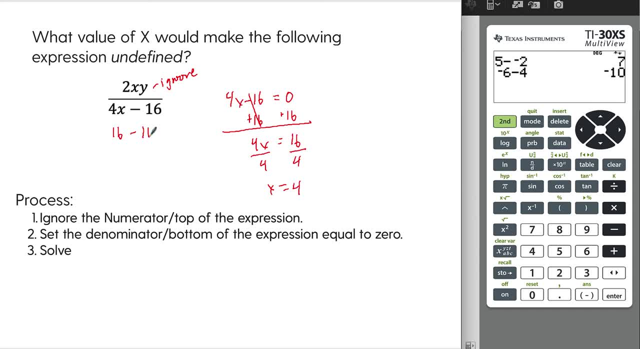 that will be 16, right. And if we can get 16 minus 16, that's zero. So how do we get 16 minus 16?? It is when x is equal to 4.. So note that x is not zero. Some students they kind of oversimplify this and they think: well. 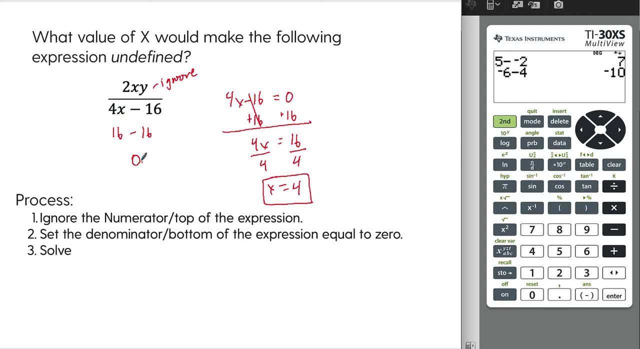 the value of x just needs to be zero and then the whole thing will be zero. If you did that, this would be zero. make that zero, but you would have negative 16 on the bottom still. Okay, so x isn't always zero. x is often some other number that makes it undefined. 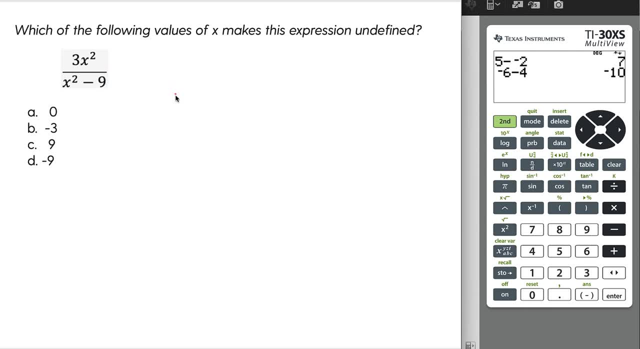 All right, so which value? which of the following values of x, makes this expression undefined? All right, so we're going to do this, We're going to do this, We're going to do this Again. ignore the top. We're not trying to solve for the whole thing, We just want this to be. 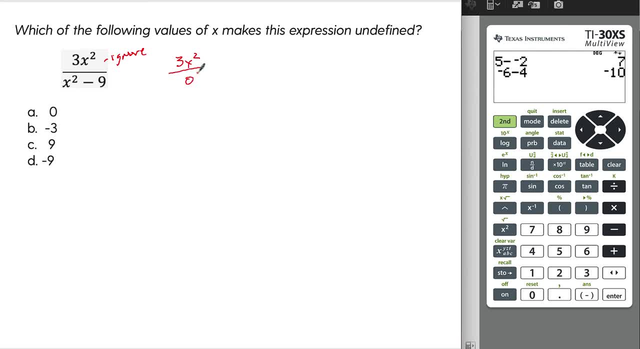 effectively 3x squared over zero. So you got multiple choice Again. if you put zero in there, you're going to get minus nine. This will be zero, but you were left with a minus nine. What we want is actually nine minus nine. That is equal to zero. So how do we get nine here? Well, 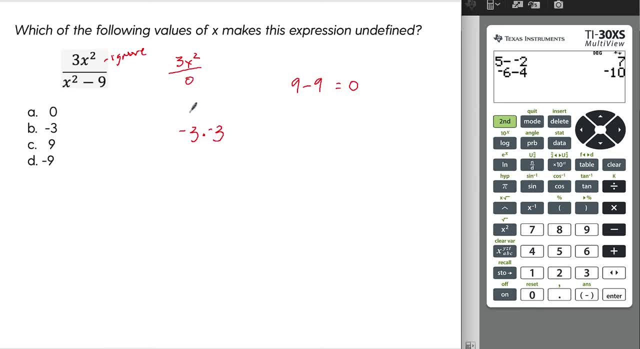 what is negative three times negative three, Because that's what x squared is. So here you would have negative three squared, which is negative three times negative three, It is nine. So this is our answer. Again, why wouldn't nine fit? Because you're squaring it and you would have nine squared. 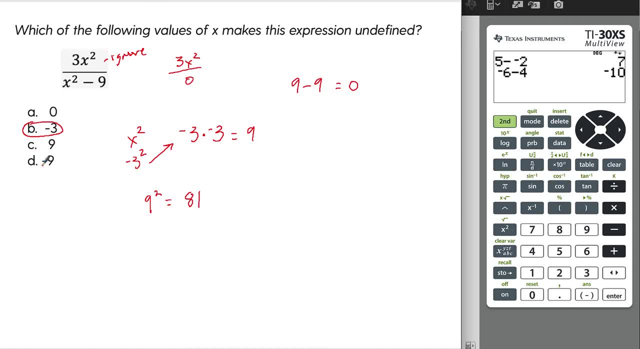 which is 81. That's why either c or d don't work. They both would be equal to 81.. What are the undefined points in this numerical expression? So again, if we can get 14, actually negative 14 plus positive 14, that is equal to zero. 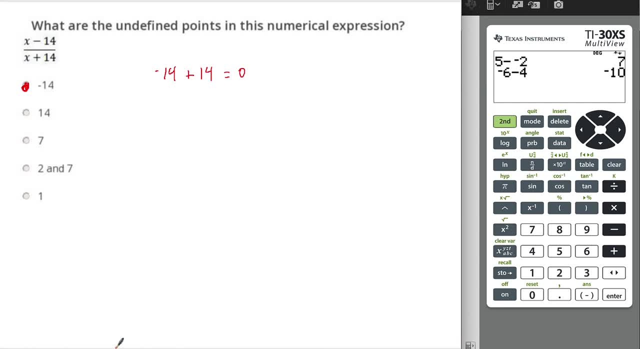 So here's our answer right here. Let's do another one. What are the undefined points in this numerical expression, Again very similar to the other one we had, but in this case it could be three or negative three. You want to look out whenever they give. 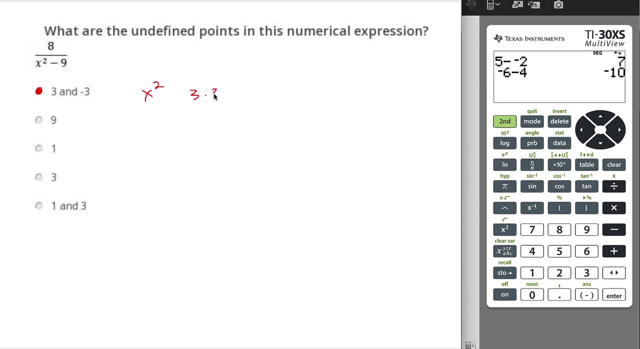 you: x squared Three times three is nine, but so is negative three times negative three, That is also nine. What are the undefined points in this numerical expression? So this one is a little bit trickier. We got seven x Again. we're going to ignore this part, though. 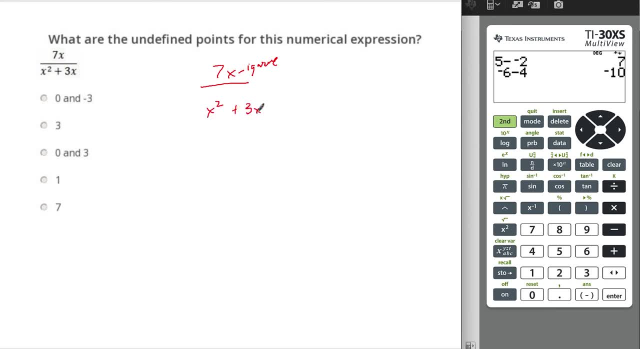 over x squared plus three x. In this case it would be best to just put in these values here. So if we put in a zero here, zero squared is zero plus three times zero is zero. Now that works. Let's see if negative three works. 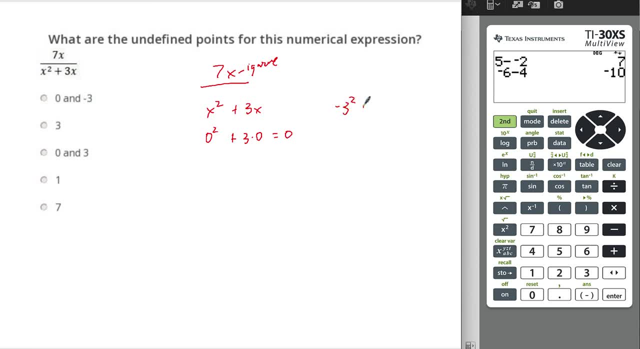 So if we do negative three squared plus three times negative three, well, negative three squared will be positive nine, but then three times Negative three is negative nine, which is zero. So this one works. Will positive three work. Will positive three work. 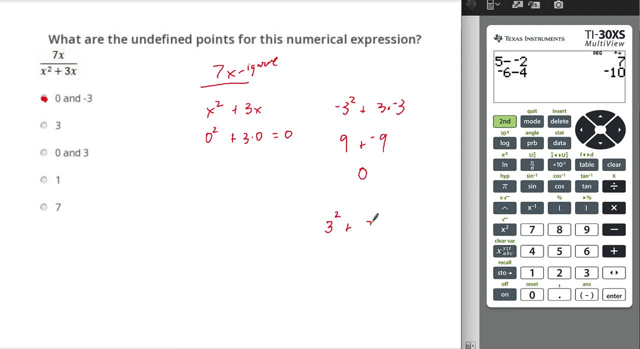 So let's look: Three squared plus three times three, Three squared is positive. nine plus three times three, which is nine, That's 18.. So you would end up with 18 on the bottom, which isn't going to make it undefined. 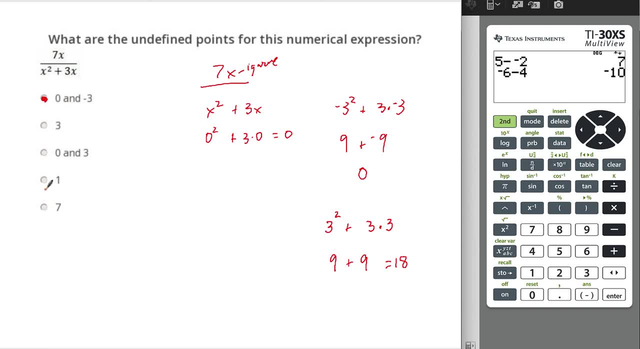 So this is the only one that works. One and seven aren't going to work. Three alone isn't going to work either. All right, There are some other examples where you would find an undefined situation. So the slope of a vertical line.